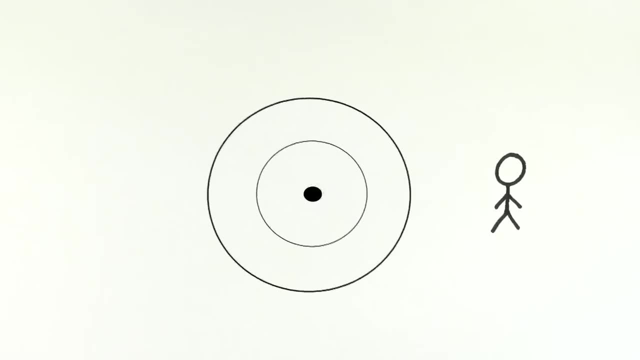 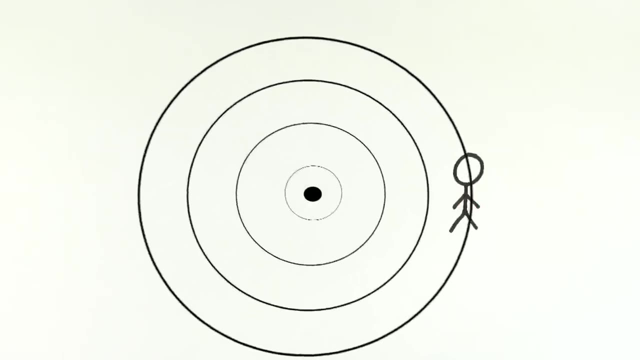 But what will happen? if you run toward the speaker, You'll hear a higher frequency because more wave crests will strike you per second. If you run away from the speaker, you'll hear a lower frequency because less wave crests will strike you per second. 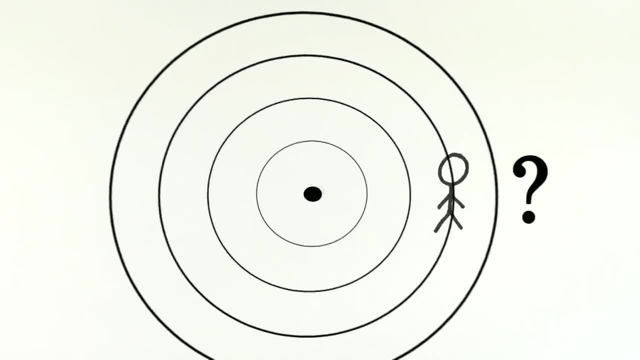 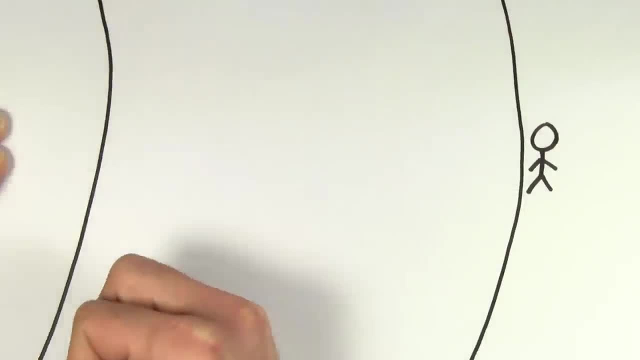 But how do we figure out exactly what frequency you'll hear? To find out, let's zoom in on what's going on. Say, a wave crest has just made it to your location. The time it takes until another wave crest hits you will be the period that you'll observe. 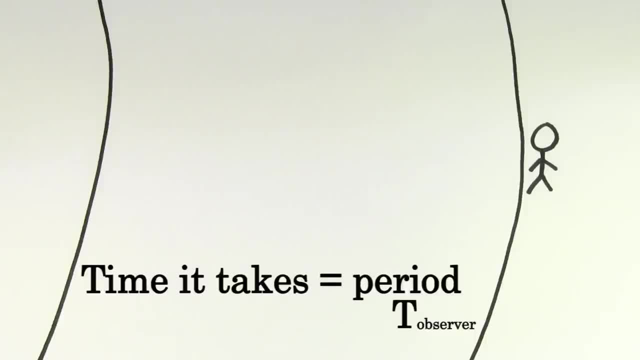 since that will be the time you observe between wave crests. If you're at rest, you'll just have to wait until another wave crest gets to your location, And the period you'd observe would be the actual period of the wave emitted by the speaker. 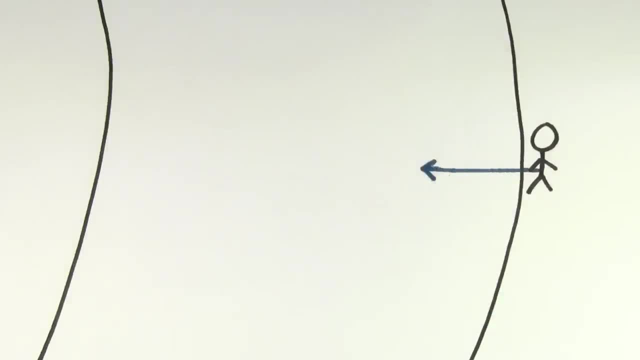 But if you're running toward the speaker or wave source, you don't have to wait as long, since you'll meet the next wave crest somewhere in between. If you can figure out how long it takes for the next crest to hit you, that would be the period that you'd observe and experience. 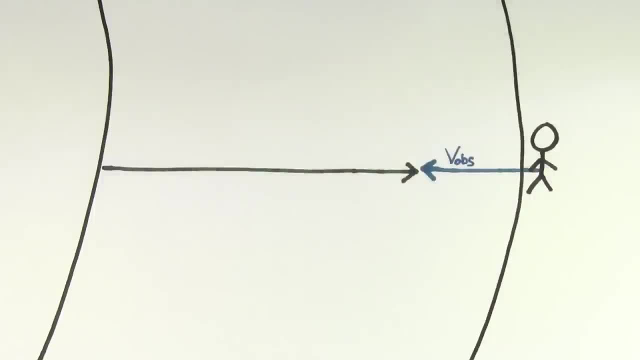 Let's say you're moving at a constant speed, that we'll call VOBS for the speed of the observer. The distance you'll travel in order to reach the next crest will be your speed times, the time required for you to get there. 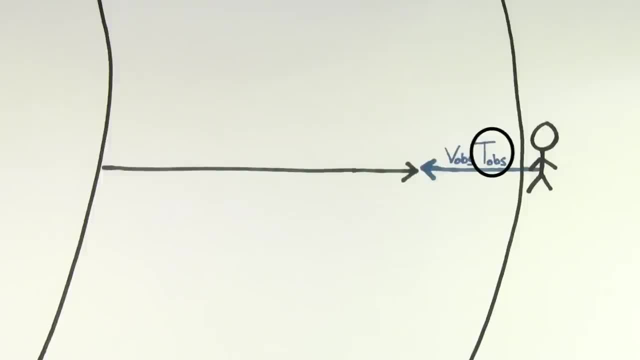 But this time is just going to be the period you observe, since it will be the time you experience between wave crests. So we'll write the time as TOBS for period of the observer. Similarly, the distance the next wave crest will travel in meeting you. 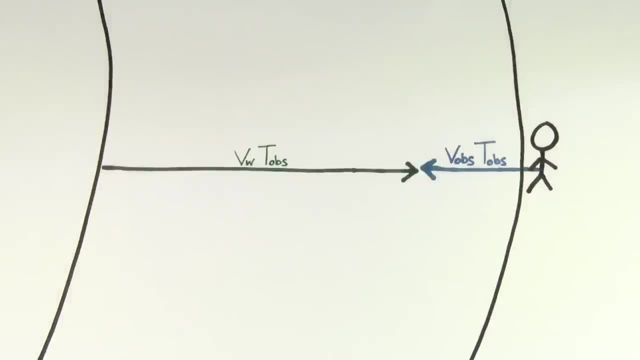 will be the speed of the wave. VW times that same amount of time, which is the period you are observing. But now, what do we do? Well, we know that the distance between you and the observer is the speed of the wave. 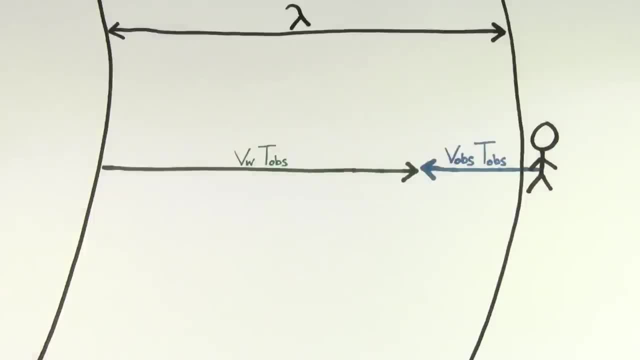 Well, we know that the distance between you and the observer is the speed of the wave. Well, we know that the distance between crests is the actual wavelength of the wave, Not the observed wavelength but the actual source wavelength emitted by the speaker at rest. 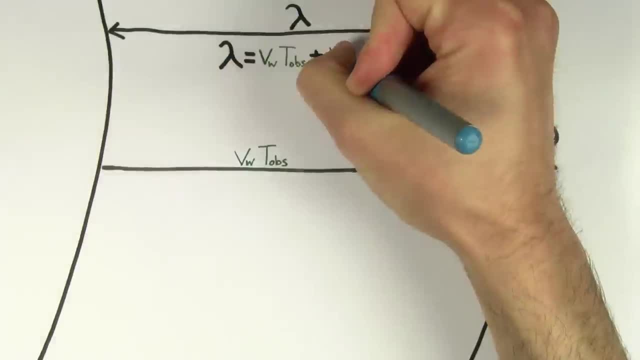 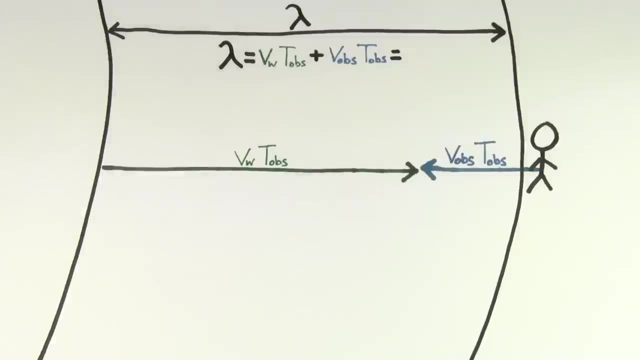 So if we add up the distance that we ran plus the distance that the next wave crest traveled to meet us, they have to equal one wavelength. in this case, We can now pull out a common factor of TOBS If we solve this for the period of the observer. 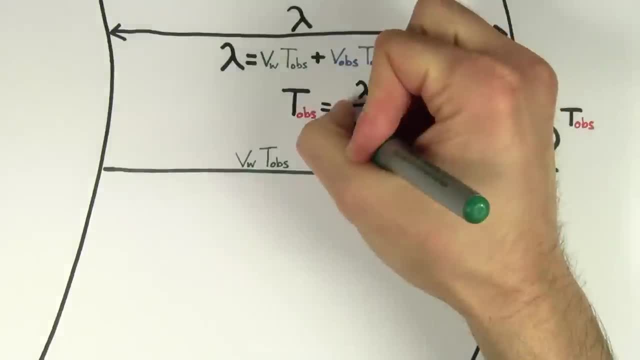 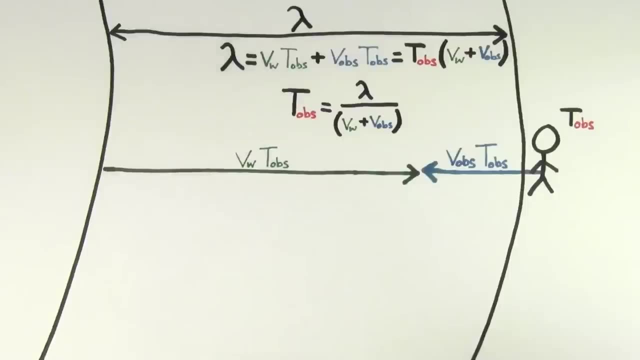 we find that it will be equal to the wavelength of the source divided by the speed of the wave plus the speed of the observer. So this is a perfectly fine equation for the period experienced by a moving observer, but one side is in terms of period and the other side is in terms of wavelength. 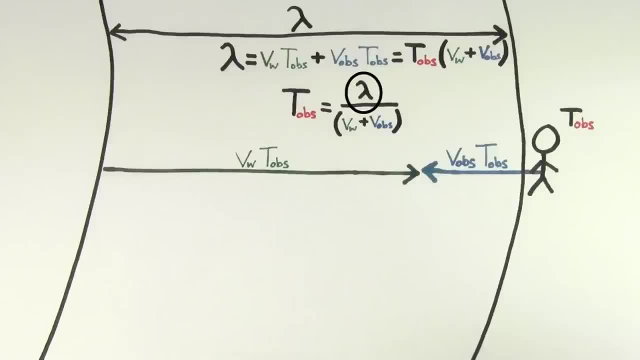 So if we want to compare apples to apples, we can put this wavelength in terms of period by using this formula: The velocity of the wave must equal the wavelength of the source divided by the period of the source, Since this wavelength was the actual wavelength emitted by the source. 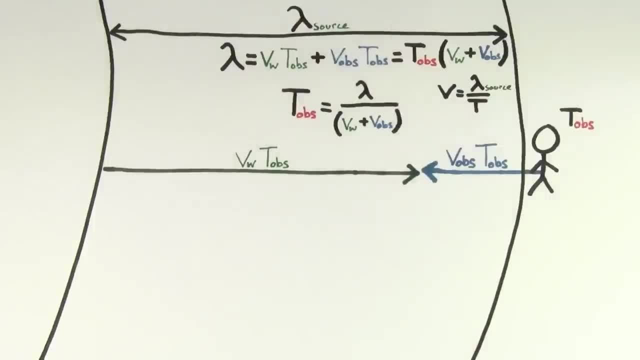 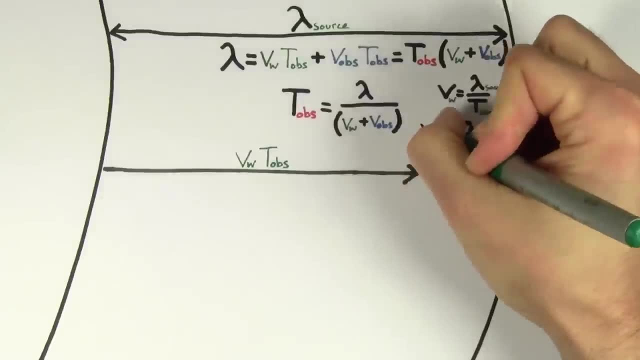 or the speaker. we have to also use the actual period emitted by the source, not the observed period. If we solve for the wavelength, we get that the speed of the wave times, the period of the source, has to be equal to the wavelength of the source. 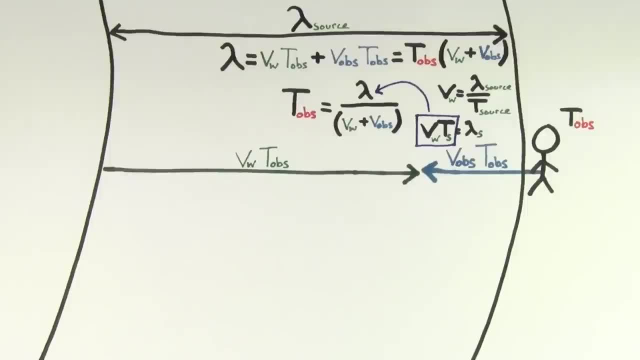 So we can plug in this expression for wavelength and we get a new equation that says that the observed period will be equal to the speed of the wave times, the period of the source divided by the speed of the wave plus the speed of the observer. 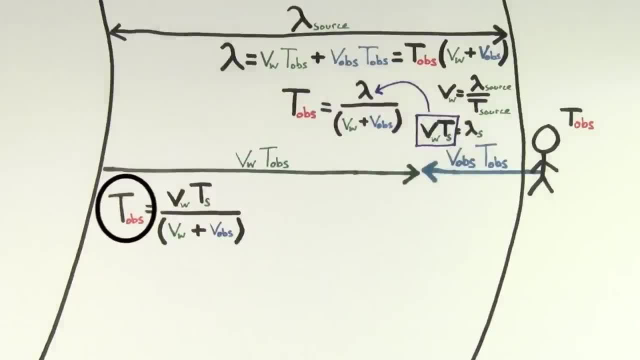 So this is a perfectly fine equation to find the observed period, but physicists and other people actually prefer talking about frequency more than period. so we can turn this statement that relates periods into a statement that relates frequencies by just inverting both sides or taking one over both sides. 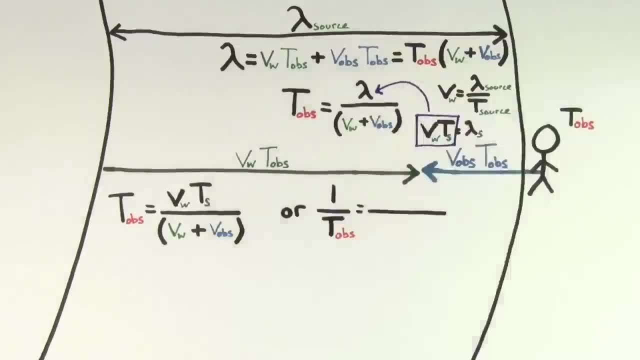 And we'll get one over. the observed period equals the speed of the wave plus the speed of the observer, divided by the speed of the wave times the period of the source. but look one over. the observed period is just the frequency experienced by the observer. 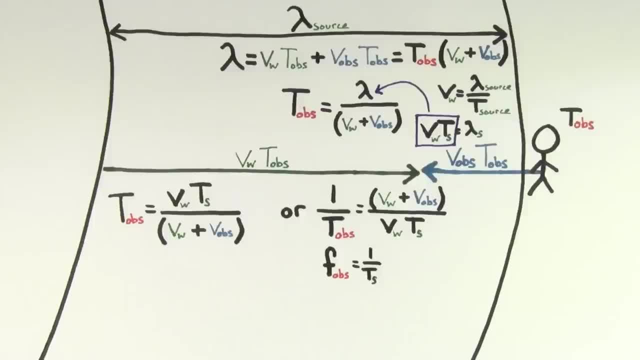 And on the right-hand side, I'm going to pull out a factor of one over the period of the source, which leaves the velocity of the wave plus the velocity of the observer divided by the velocity of the wave. And for the final step, we can put this entirely in terms of frequencies.